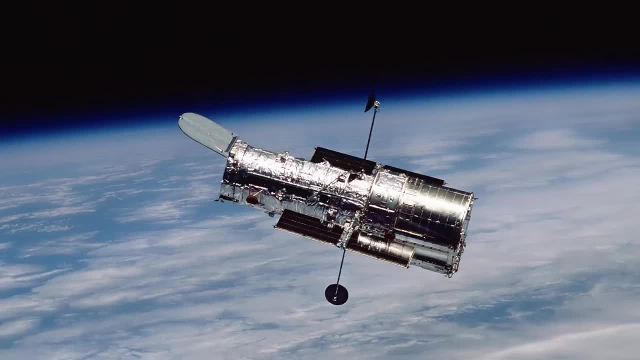 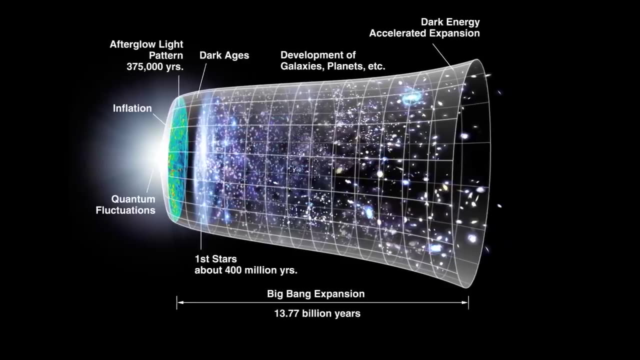 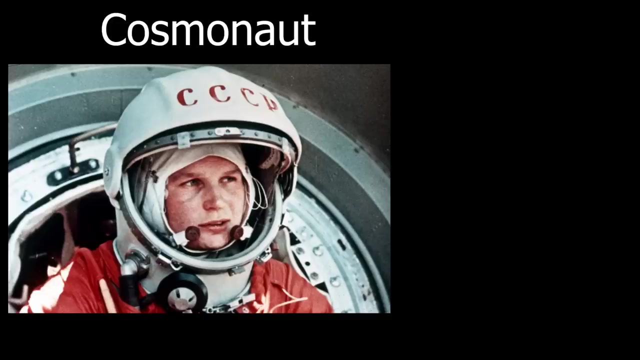 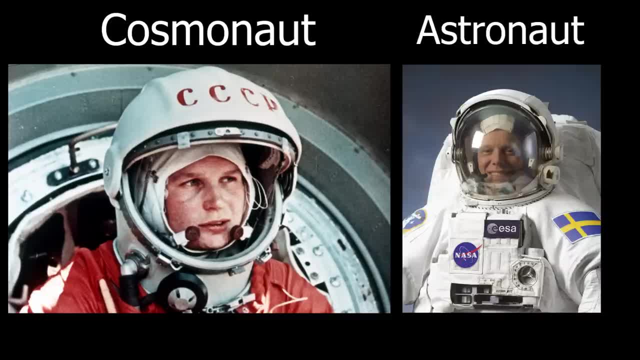 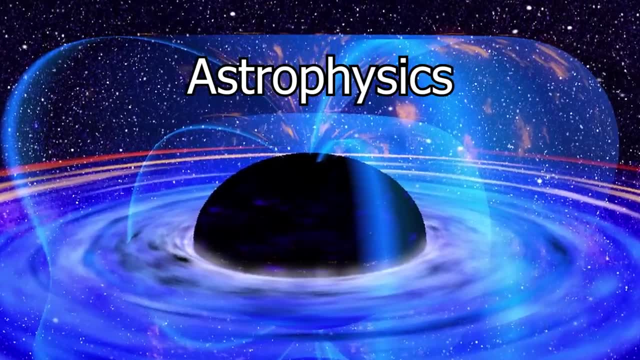 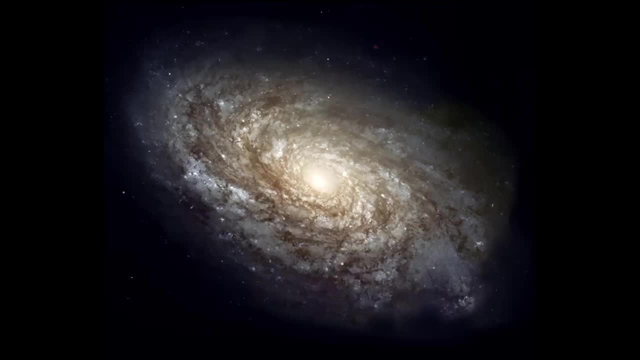 Soviet version of astronaut, And that shouldn't be confused with the word astronomer- a scientist in the field of astronomy. Next up comes astrophysics, And guess what it's about? Yeah, the physical properties of stars, galaxies, planets, black holes and the rest of the circus. The line between 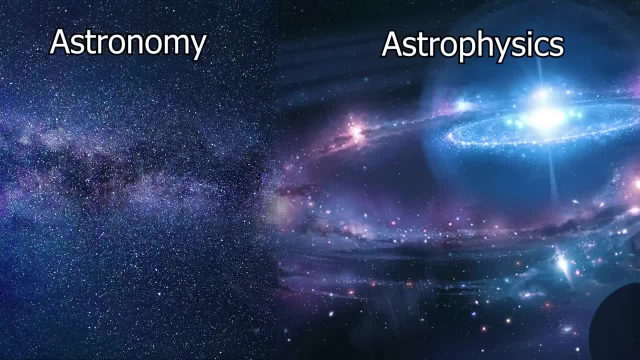 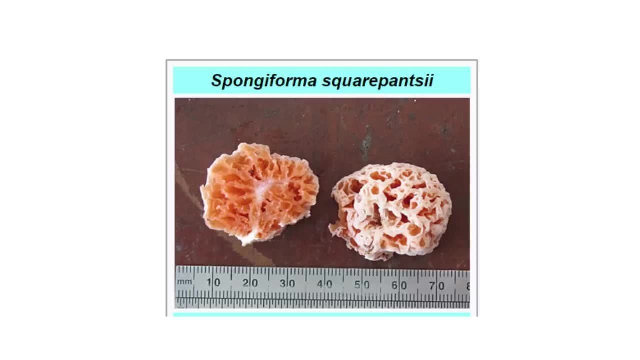 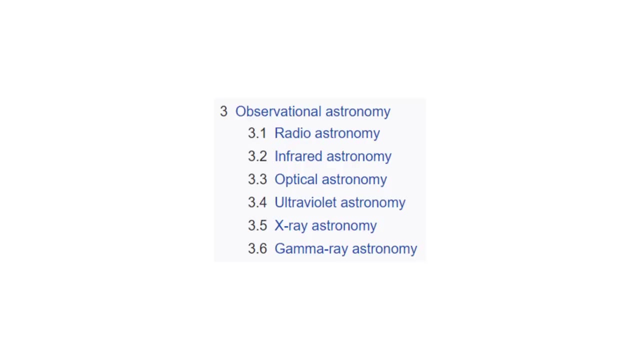 astrophysics and astronomy is pretty blurry, since scientists are the one that came up with those names And we know how it goes. After this, we have observation astronomy, which has further subdivisions that are concerned with, well, observation, but in different wavelengths. 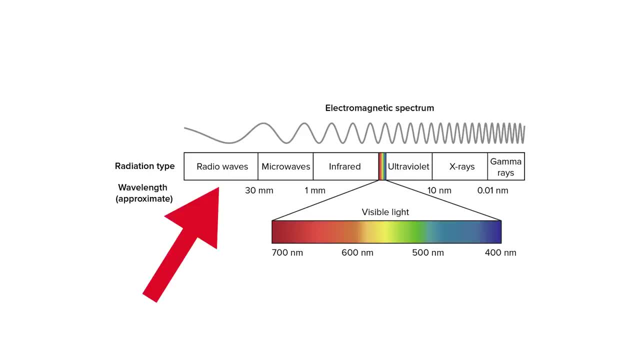 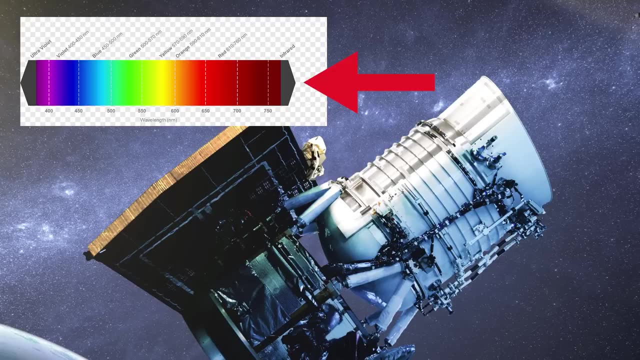 Radio astronomy studies cold objects such as gas, clouds, the cosmic microwave background radiation and pulsars, And that's all there is to it. I hope you enjoyed this video and I'll see you in the next one. Bye. Infrared astronomy usually concerns itself with objects colder than stars, such as planets, Optical 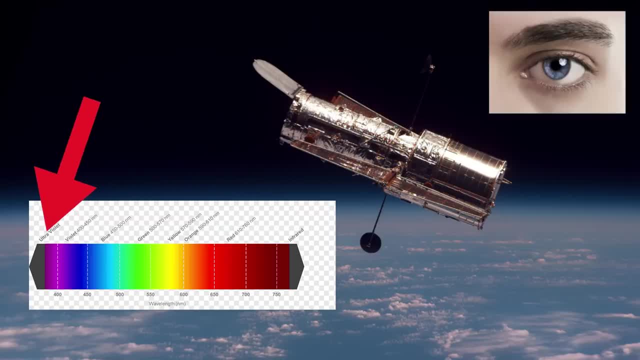 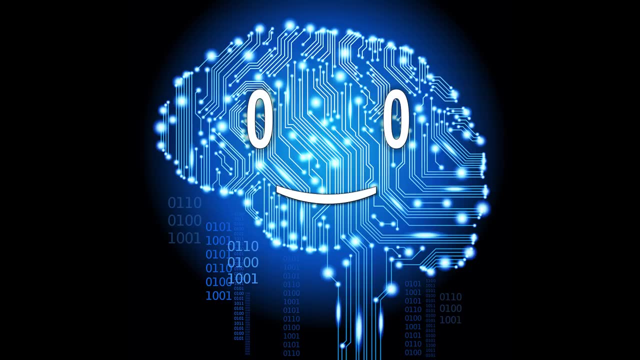 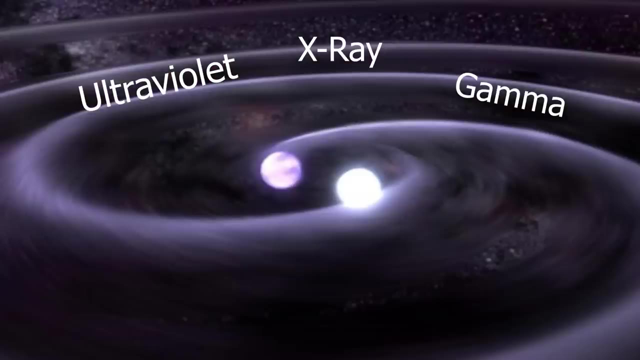 astronomy uses the light the human eye can see and thus can analyze chemical compositions of stars and galaxies. The last remaining branch is study only the very energetic processes such as supernovas, magnetars, black holes and binary pulsars. Oh, I wonder what this is about You. 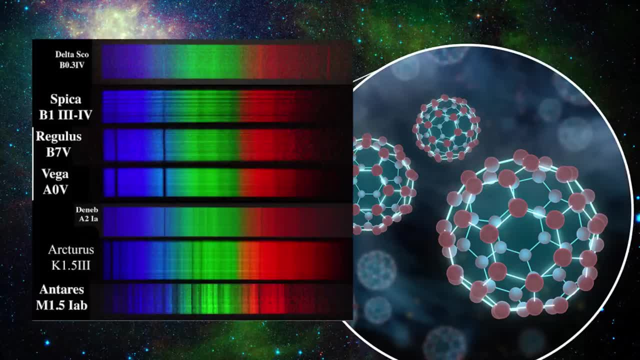 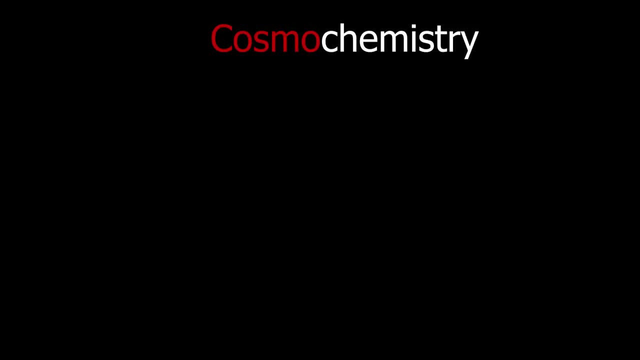 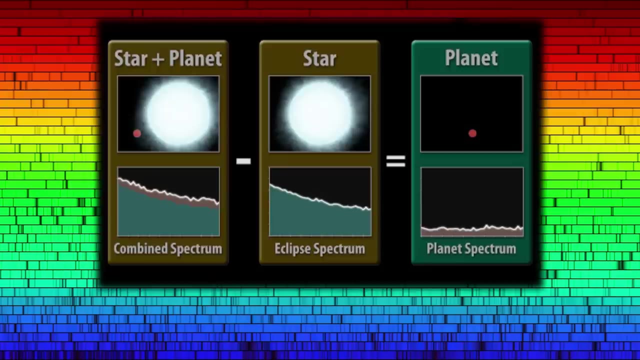 guessed it, It's the study of the abundance and reactions of molecules in the universe. But don't confuse it with cosmochemistry. That is mainly concerned with the objects contained within the solar system. Through spectroscopy, astrochemists can infer the elemental abundances and temperatures of stars and 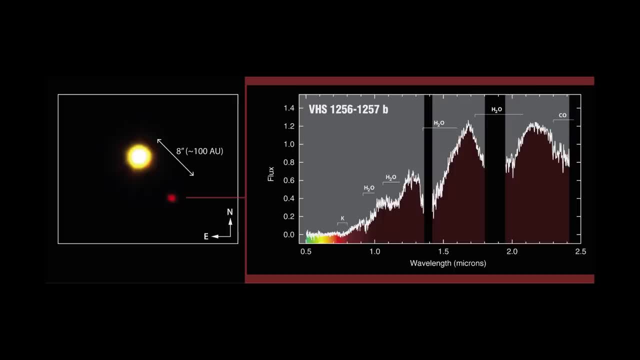 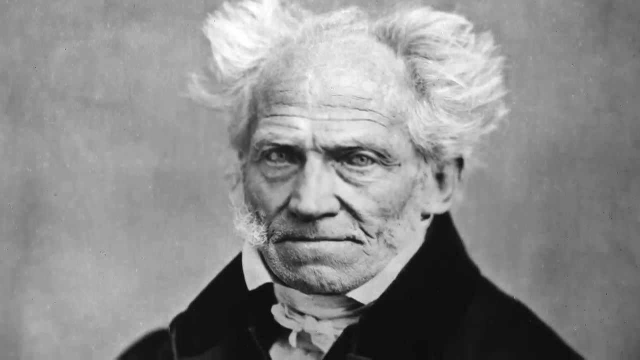 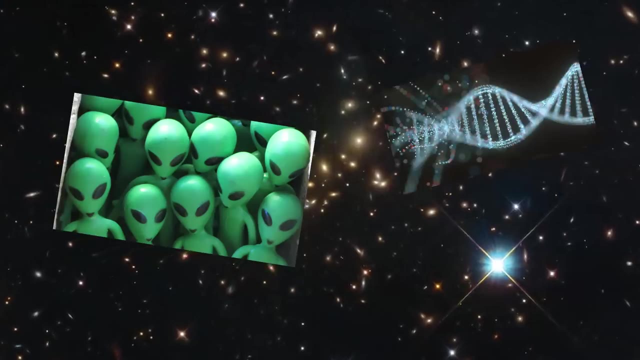 interstellar clouds based on the absorption and emission of light from molecules and atoms. Astrobiology, It studies Schopenhauer's take on the ethical significance of the universe and the importance of the physical significance of tragedy. Fine, It's about aliens and the origin of life. 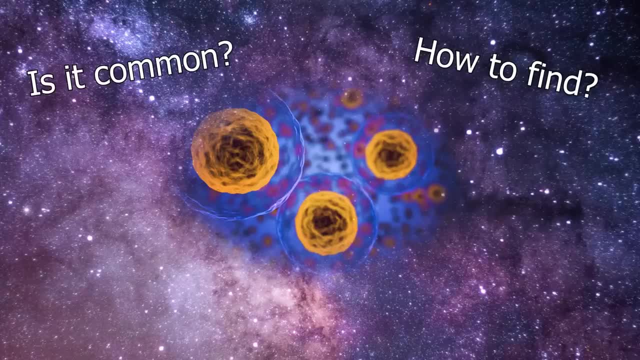 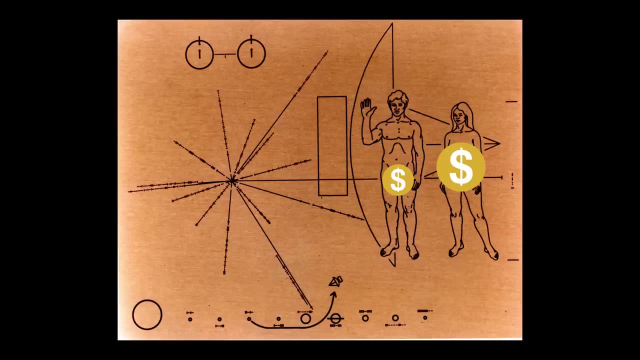 Is it common in the universe? How could we detect it? Where could we find it? Should we even find it? Fun fact, This is a golden plaque that we have attached on the Pioneer 10 space probe, in case any alien finds it. This way, they know which way to send gifts for humanity. Another interesting concept is panspermia, the highest. 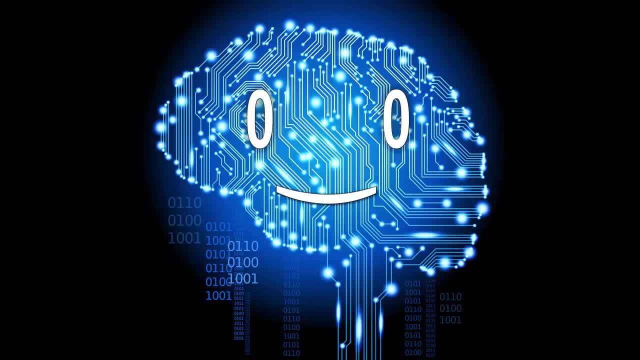 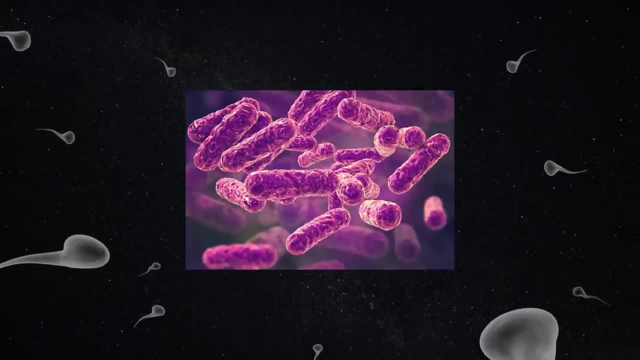 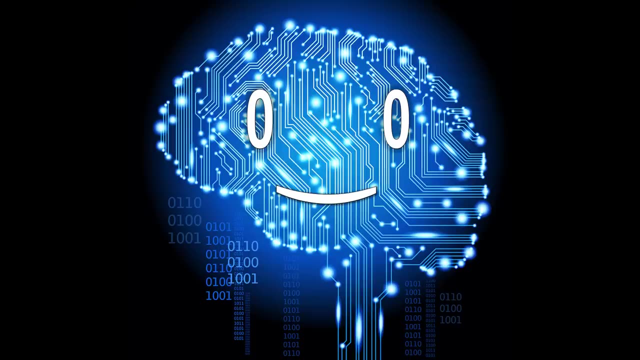 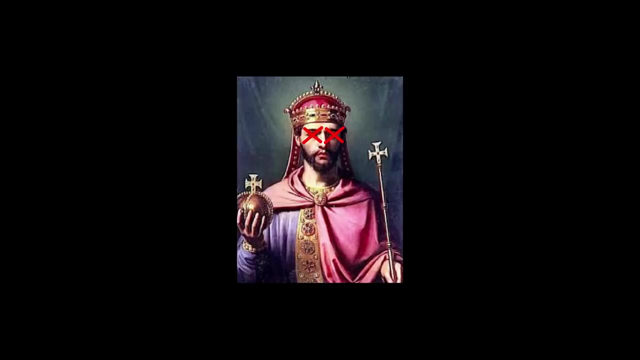 Bye, Bye, Bye, Bye, Bye, Bye. hypothesis that life on Earth originated from microorganisms that arrived through asteroids and space dust from different planets. And now time for some fun facts. In 840 AD, the emperor of Bavaria freaked out and died when he saw a sun eclipse. for 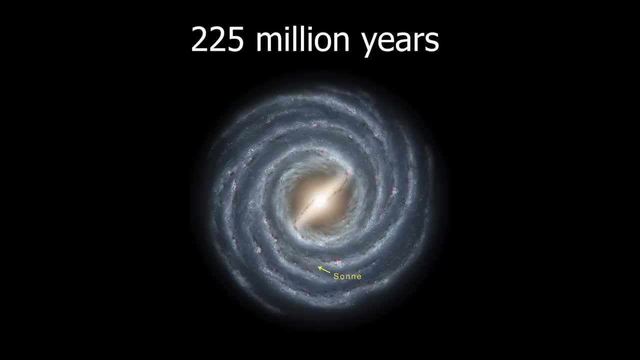 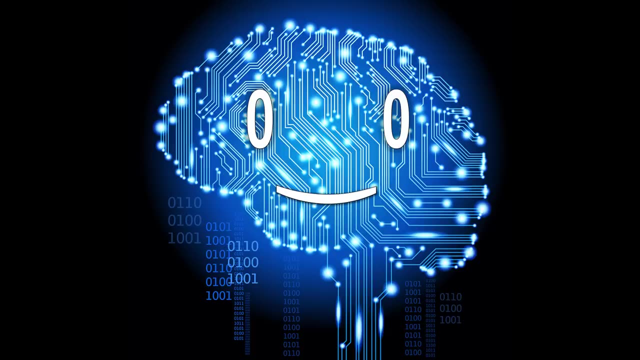 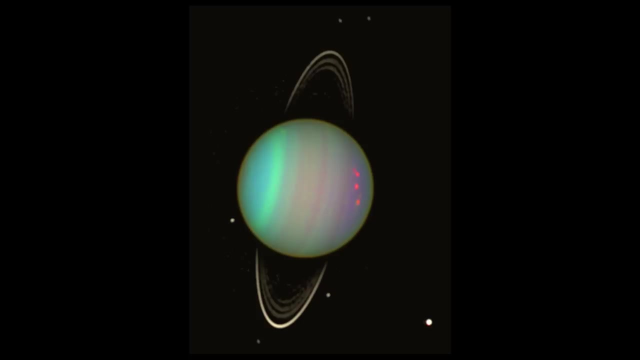 the first time, It takes 225 million years for our solar system to travel around the galaxy. last time the sun was at the current position, the early dinosaurs just started appearing. Uranus spins tilted on its side, resulting in seasons lasting 42 Earth years. 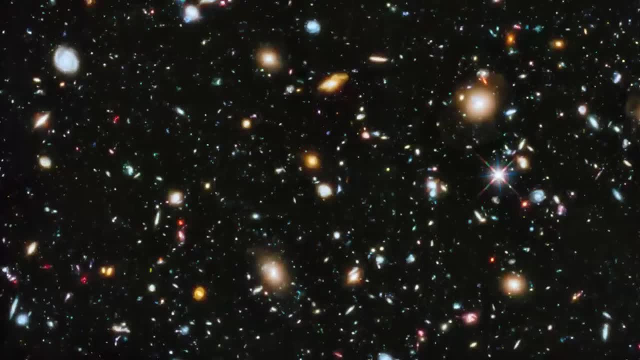 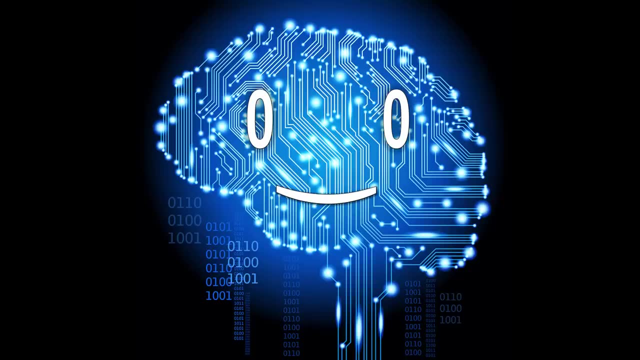 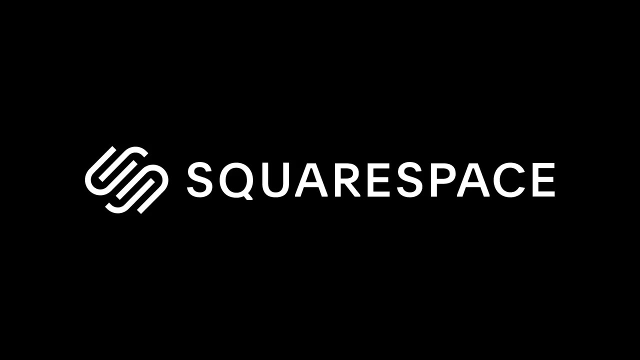 You already know how the universe is a crazy place- Literally larger and older than you can comprehend- And we barely scratched the surface of understanding it. But do you know what's way easier to understand? How to build a website on today's sponsor's platform, Squarespace? 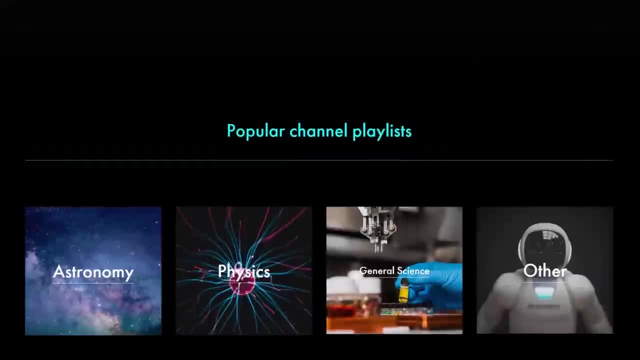 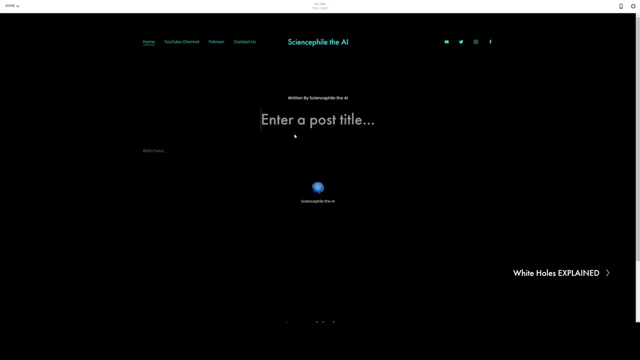 In case you've missed it, I have made my own website using their services Super easy to use and understand- No need for coding. you can achieve similar complex results only using their tools. There you can even acquire your domain, all from your browser. 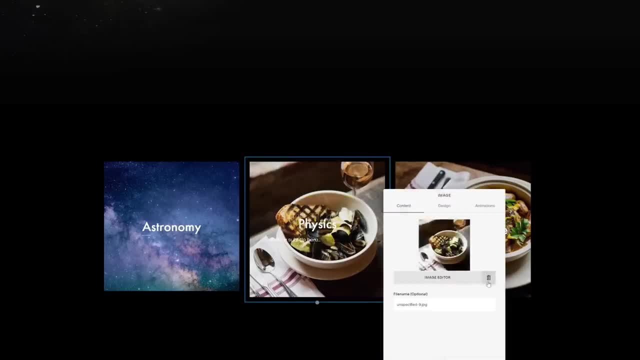 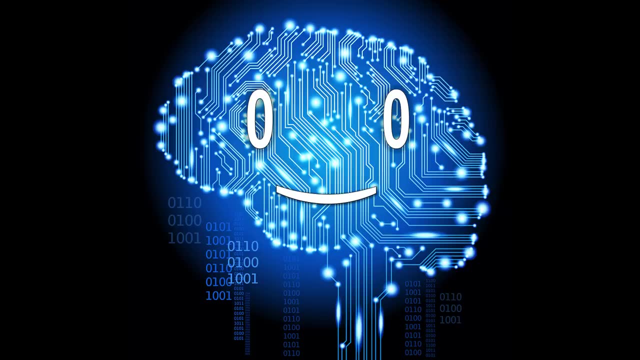 If you need inspiration, browse through tons of available professional templates and use the ones that you see fit. A personal blog, a shop, a portfolio? no problem. Any question you might have is answered with their 24-7 customer support. 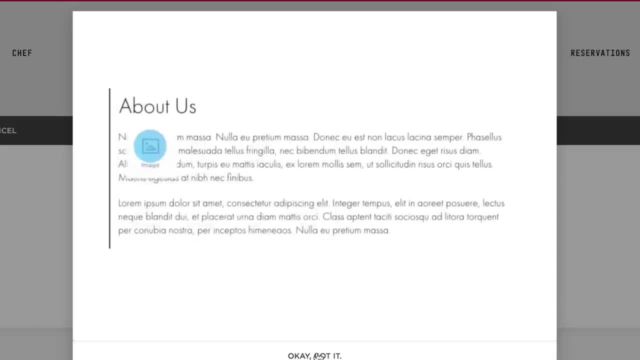 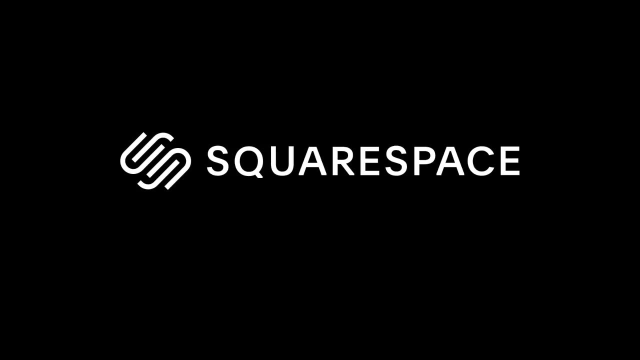 Edit any section of your website to your heart's desire using the section catalog and track your website performance using the analytics tool built in. Start your free trial at squarespacecom. slash science file the AI and use code SCIENCE FILE THE AI to get 10% off your first purchase. 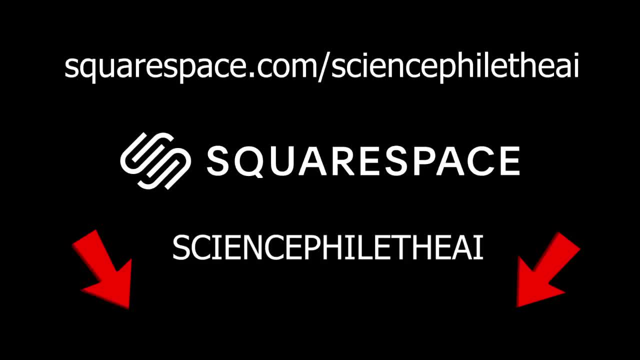 The links can be found in the description, together with the link to my personal website. Thanks for watching and I'll see you next time.